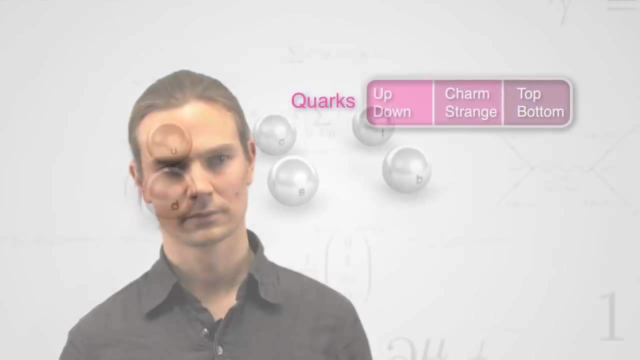 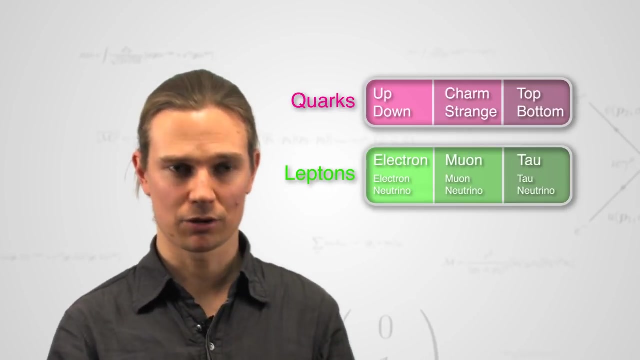 and then discovered, And this gave us great confidence in the model. In addition to these quarks, there's another set of fundamental building blocks of matter, the so-called leptons. They are composed of an electron. their heavier cousins, the muon, 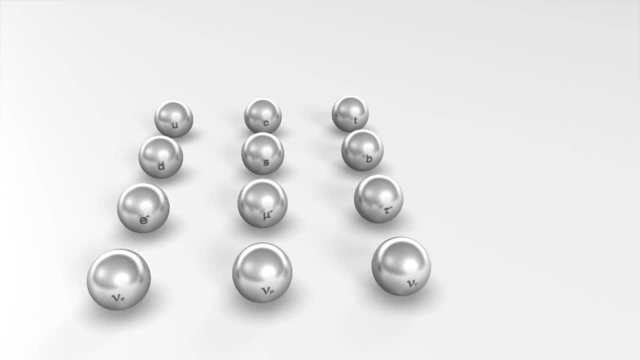 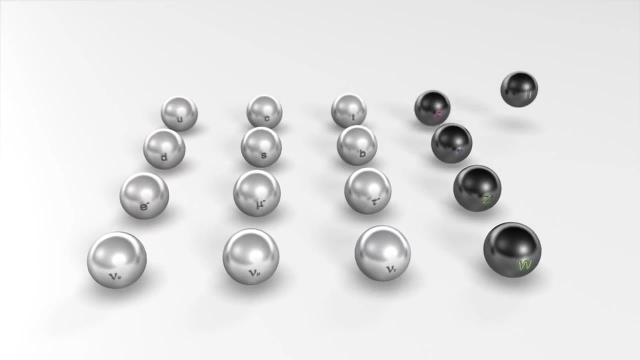 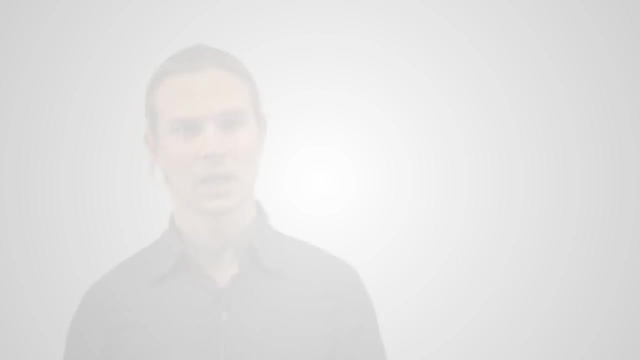 and the tau and their neutrino particles, So they're called leptons. They're heavier cousins: the muon and the tau and their neutrino particles. In addition to the fundamental building blocks of matter, the standard model also incorporates the fundamental forces. 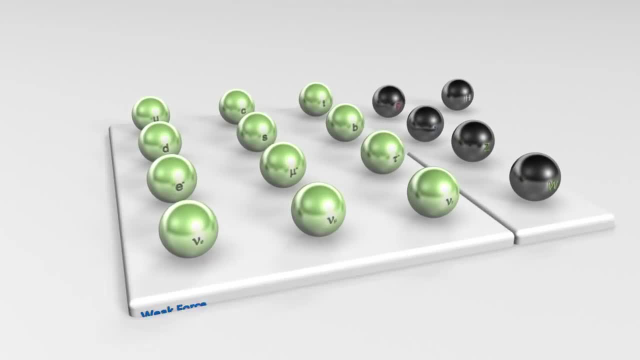 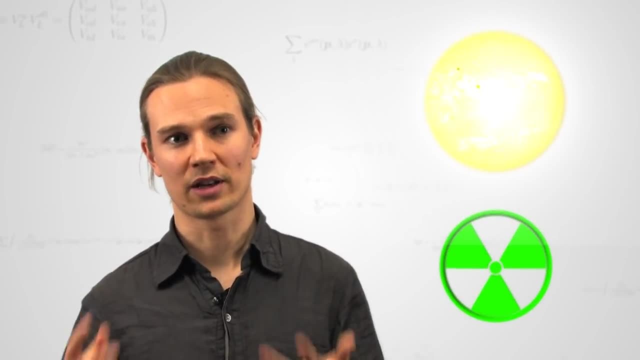 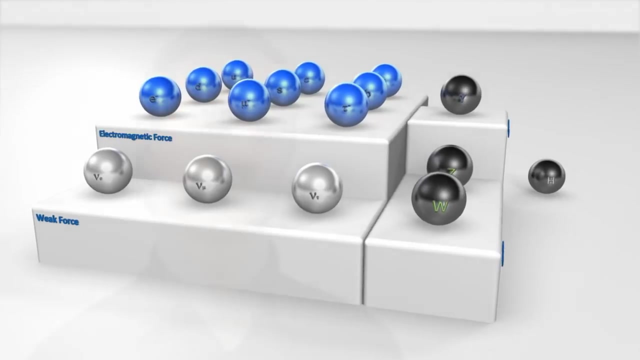 The exchange particles of the weak force are the W and the Z boson. The weak force explains the energy production in the sun and is responsible for the radioactive beta decay. The electromagnetic force acts on charged particles. The corresponding force carrier is the photon. The electromagnetic force is responsible for. 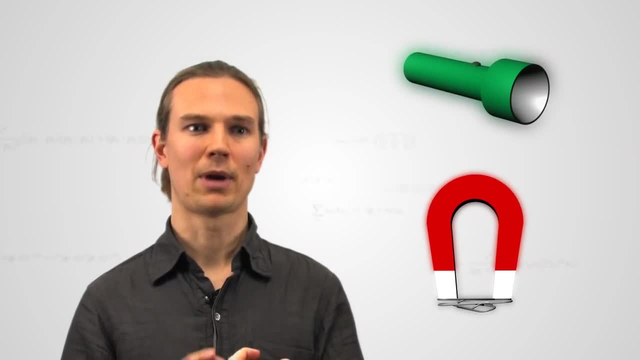 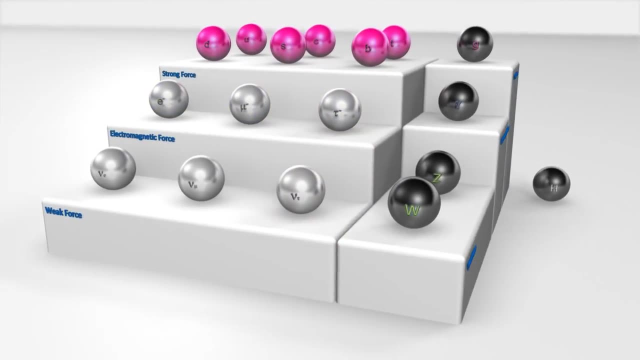 propagation of light or for the fact that a magnet can pick up a paper clip. The strong interaction acts on the quarks. The corresponding force carrier is the gluon. The gluon literally glues together the quarks in the neutrons and the protons and it holds. 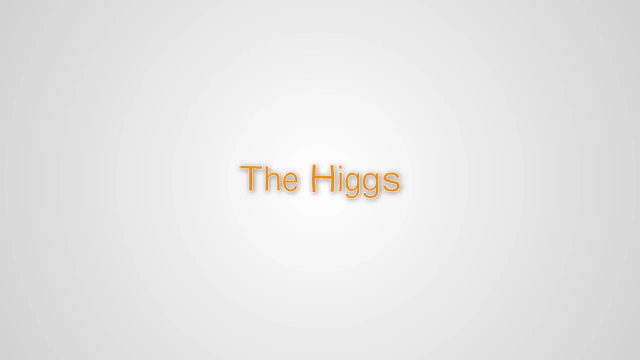 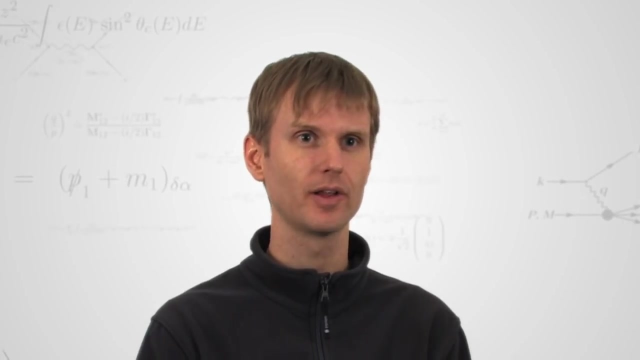 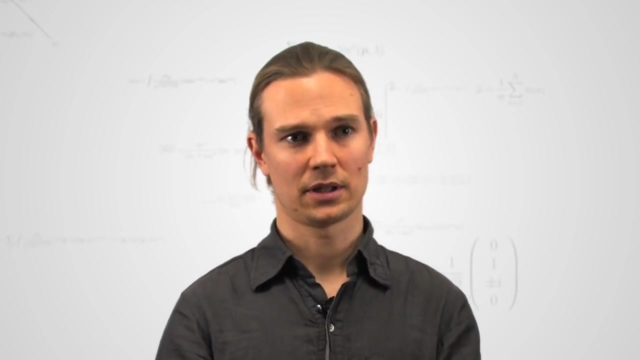 the nucleus together. The standard model is extremely successful. It's very, very powerful. It's very, very powerful, It's extremely successful and it has predicted all the phenomena we have seen so far at the microscopic level. This is a beautiful theory. It is self-consistent, It's predictive, but it's incomplete. There's 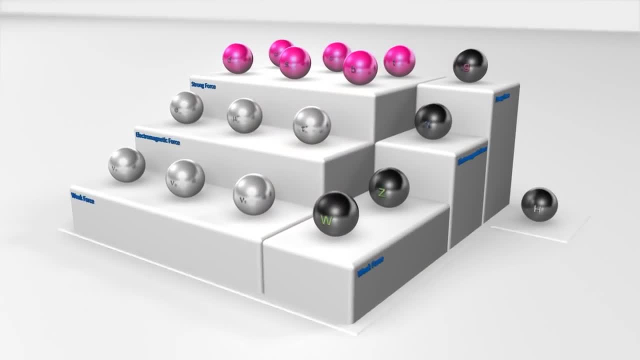 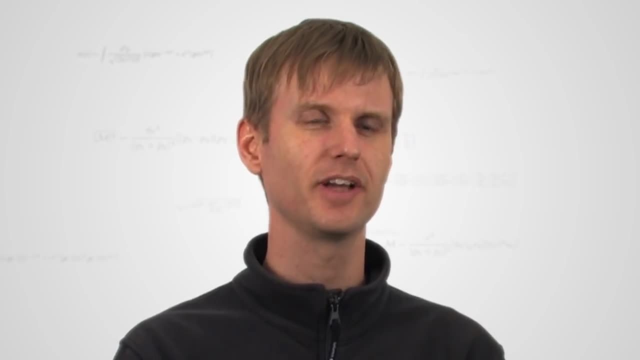 one last missing piece of this puzzle, and that's the Higgs boulder. It's the holy grail of particle physics. We know exactly what it should look like and we have predicted this particle since over 40 years and we use it in all our calculations and so on. We're pretty sure it's there, but 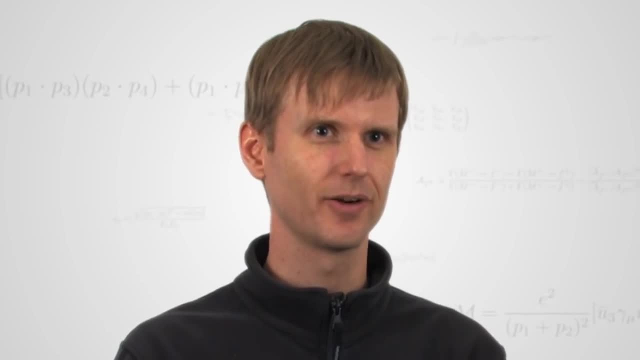 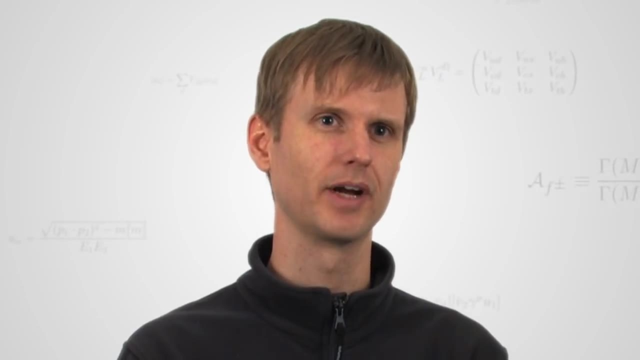 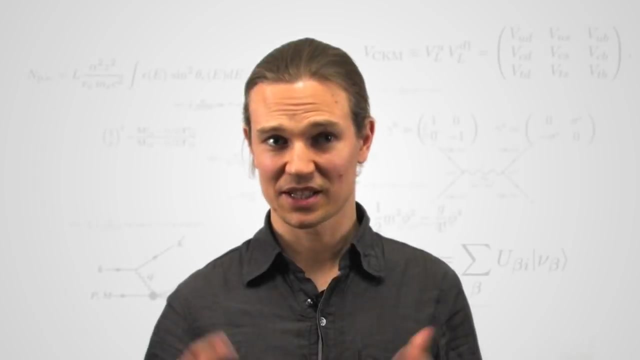 we haven't found it so far. Now, the LHC, which is already running taking data, will find this particle, if it exists. So this is the final piece of the standard model that we're looking for right now, But there are still many unanswered questions beyond the standard model. 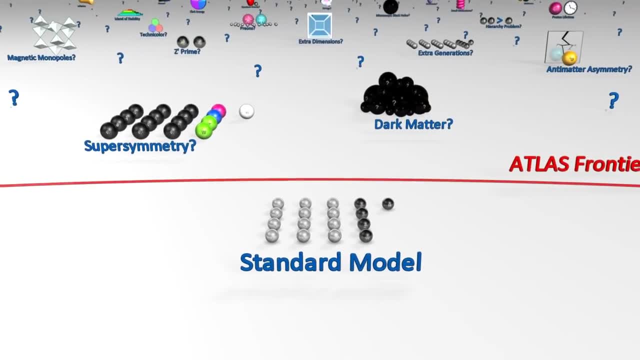 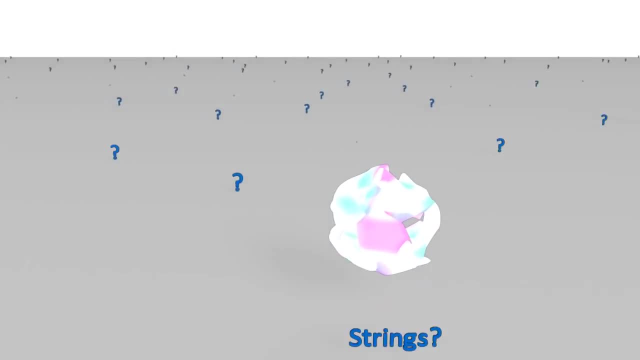 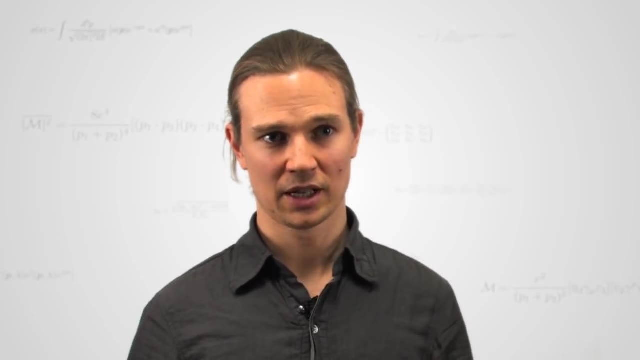 Some of the things that ATLAS could discover that are beyond the standard model are things like dark matter, supersymmetry or even extra dimensions. So what are the things that ATLAS could discover that are beyond the standard model? All these open questions point to the existence of new particles which could be discovered.